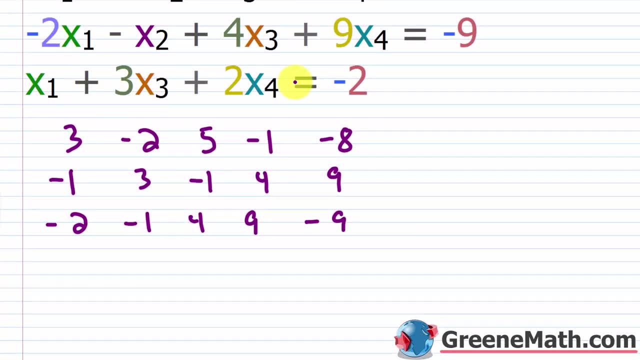 better and let me scroll down a little bit. Then, in this last equation, I want you to notice that you don't have an x sub 2.. Whenever you're missing a variable, you want to write a 0 as the coefficient for that variable to act as a placeholder. So I'm going to put a 1 and then 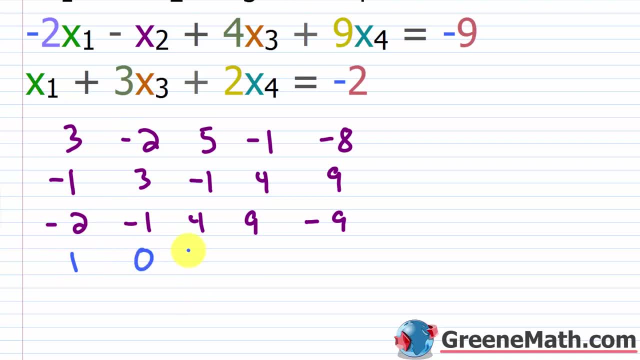 again, for my x sub 2, I'm putting a 0 as the coefficient. Then for x sub 3, I put a 3, then my 2, then my negative 2.. Okay, so this guy is now set up for us and we are ready to go. So let me copy this real quick Now, the quickest way. 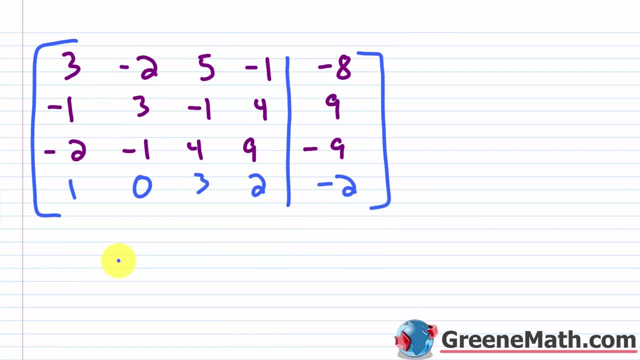 to solve this if you only know kind of Gaussian elimination or Gauss-Jordan elimination. if you just get this, and this is where you are in your chapter, I would suggest just doing the Gaussian elimination, putting this matrix in row echelon form, meaning I'm just going 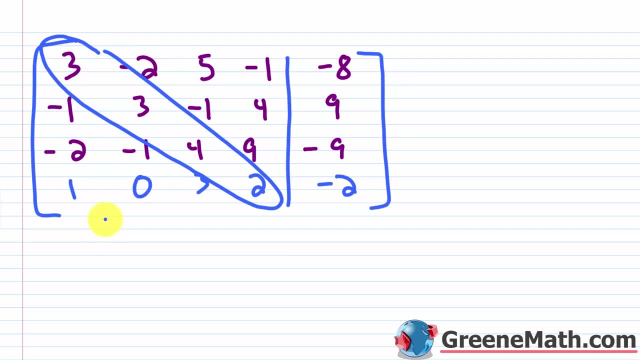 to get 1s down the diagonal and 0s below the diagonal. It's going to be really quick to do that and then kind of back substitute to get your answer. If you go through to reduced row echelon form again, that's from the Gauss-Jordan elimination. 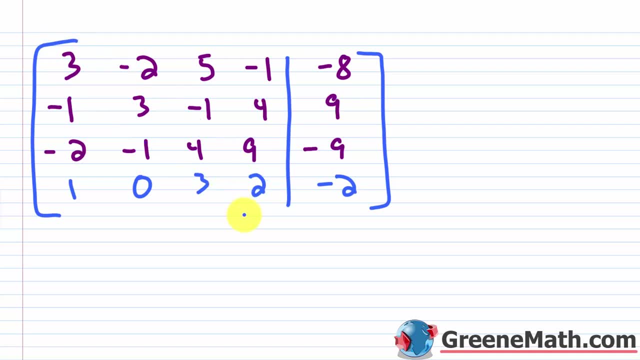 it does take a little bit longer. That is what we're going to do today, just to get a lot of practice on the elementary row operations, because I feel like you do need it. It's just something that comes up, it goes away and then later on if you have to go back to it, 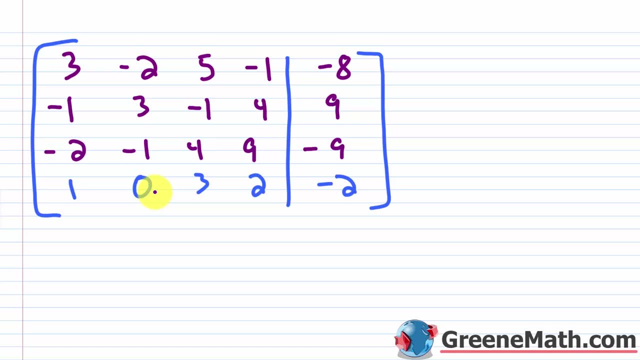 it's something. if you didn't practice enough, you kind of forget it and then you might struggle with it again. Alright, so the very first thing I want to do is I want to get a 1 as this top position here, and then I want to work below and get 0s Every. 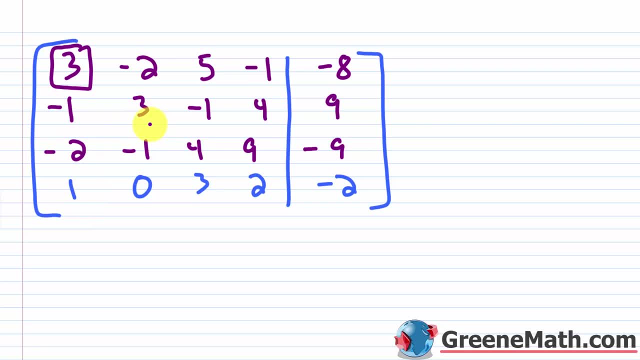 time I go to the right, to a new column, I want to get my 1 first and then my 0s. So what I'm going to do, I could multiply this first row, which I'd label as row 1.. Let me label. 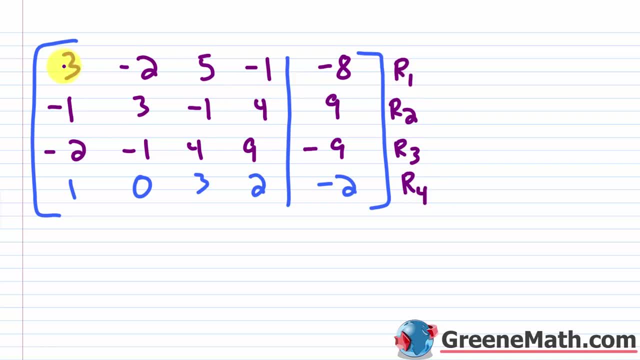 all these real quick. I could multiply row 1 by 1 third. but there's an easier solution. Remember, for the elementary row operations I can swap two rows So I can say row 1 is with row 4 because I already have a 1 there. and if I swapped those rows this guy would 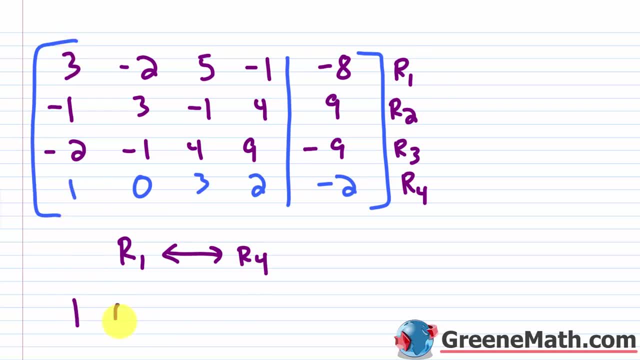 come up here. So let me just write this real quick. I have 1,, 0,, 3,, 2, and negative 2.. I'll just erase this from here. I'll just copy this here: 3, negative, 2,, 5, negative, 1, negative 8 and. 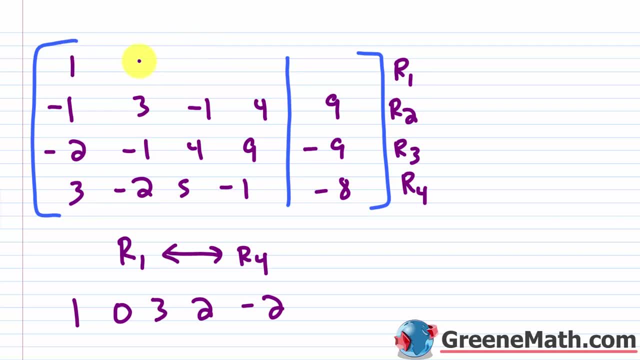 then I'll just copy this right here: So 1, 0,, 3,, 2, and negative 2.. Okay, so now that I have my 1 in this position here, These rows are being changed. You can see that I'm not. going to change anything. The rows are being changed. I'm going to just do the same thing. I'm going to do the same thing over here. I'm going to say row 1,, 0,, 3,, 2, and negative 2.. I'm going to. 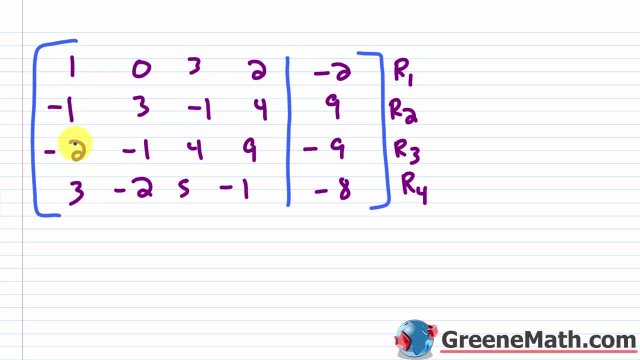 ones going down are pretty easy to get, and I'm going to do multiple ones at once. okay, we're ready to kind of speed up this process. so we know that if we want this to be a zero, I've got to add the opposite of that number to it. okay, so in this case, I've got to add a one. in this case, I've got. 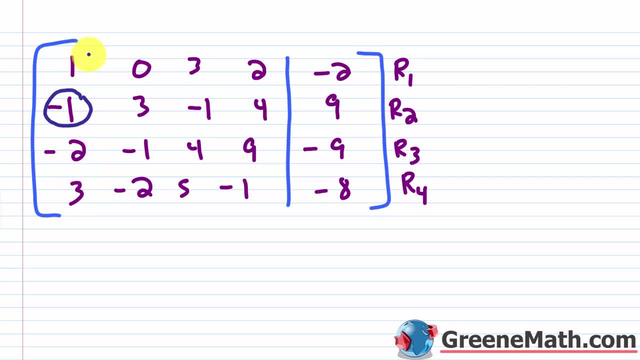 to add a two, and in this case I've got to add a negative three. well, this one is really convenient, because whatever I multiply by one, it's just itself. so what I'm going to do in each case is I'm going to multiply row one by whatever I need to add to this to make it a zero, and then I'm going. 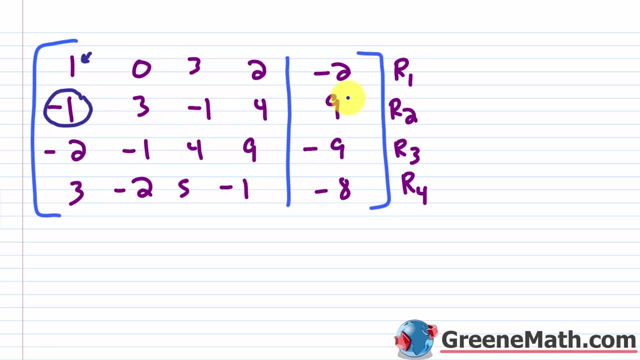 to add it to that row and then that's what I'm going to replace the row with. okay. so for the first one, I'm going to say that I'm going to have one times row one plus row two. this is what I'm going to replace row two with, okay, and when you multiply something by one, it's just itself. so 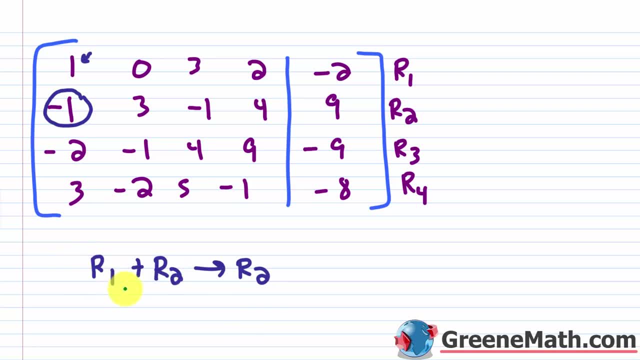 really you could just say row one plus row two. if you want, then for the next one I'm going to end up saying that I'm going to have two times row one. okay, so the opposite of negative two is two. so two times row one plus row three. 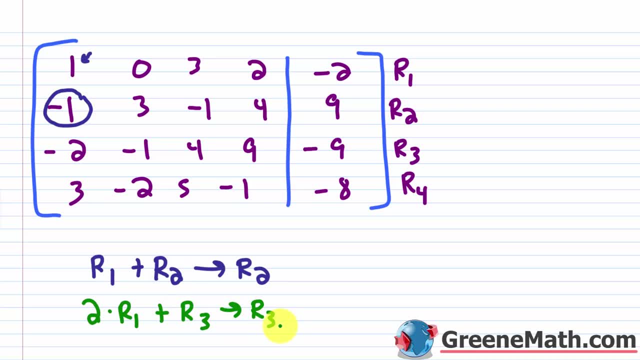 that's what I'm going to replace row three with. and then, for this last one here, I'm going to have negative three. okay, because negative three plus three is zero. so negative three times row one plus my row four is what I'm going to replace row four with, okay, so let's go through and crank. 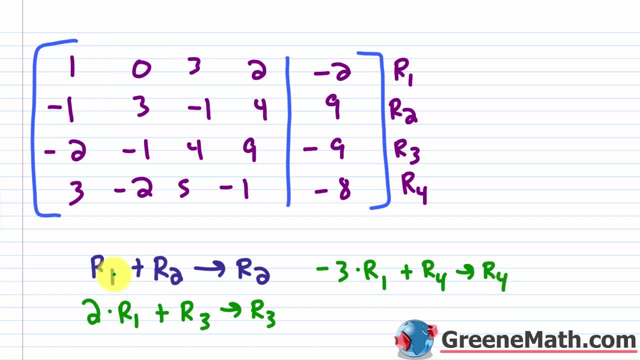 this out real quick. so I know, for this one I'm just adding row one and row two. that's what I'm replacing row two with. so one plus negative one is zero. zero plus three is three. three plus negative one is two. two plus four is six and negative two plus nine is seven. so this: 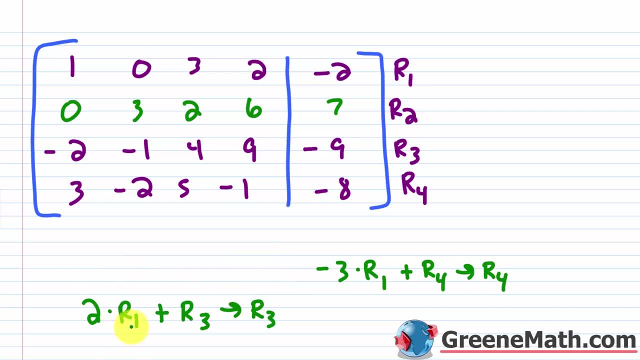 one is done, then for this one two times row one plus row three. that's what I'm going to replace row three with. so two times one is two. two plus negative two is zero. two times zero. zero. zero plus negative one is negative one. then two times three is six. six plus four is ten. two times two is four. four plus nine is thirteen. 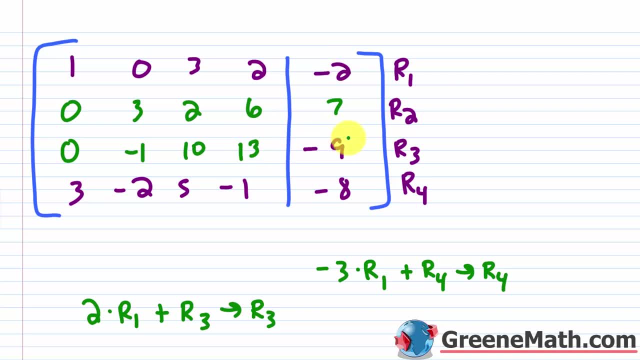 two times negative. two is negative. four negative: four plus negative. nine is negative thirteen. all right, so this one is done. so let's do this one. so we have negative three times row one plus row four, negative three times. one is negative. three plus three is zero. we know that this would 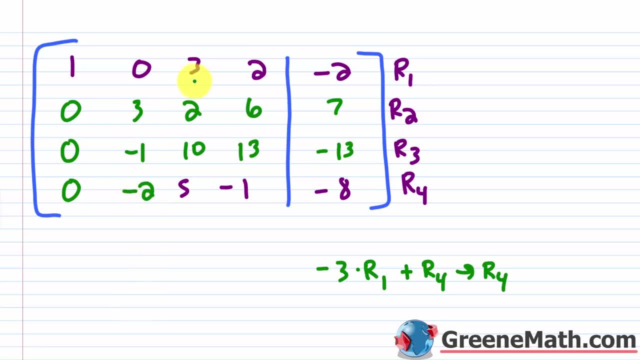 be still negative. two. negative three times three is negative nine. negative nine plus five is negative four, and then negative three times two is negative six. negative six plus negative one is negative seven. then, lastly, we have negative three times negative two, which is going to be positive six. 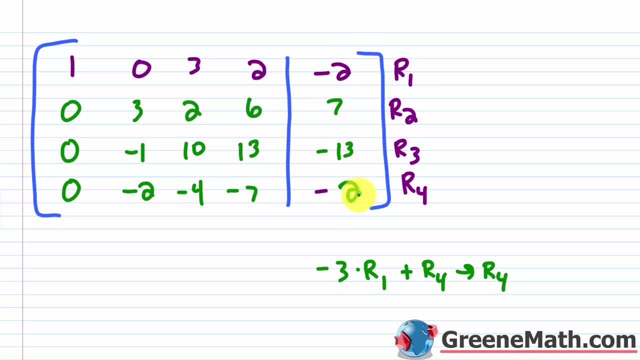 and then positive six plus negative eight is negative two. all right, so that part's done. I have a one here and zeros below. now I want to move to my next column and I want to get a one here. okay, I already have a zero above, so I'm going to get that one first, and then I'm going to get the zeros. 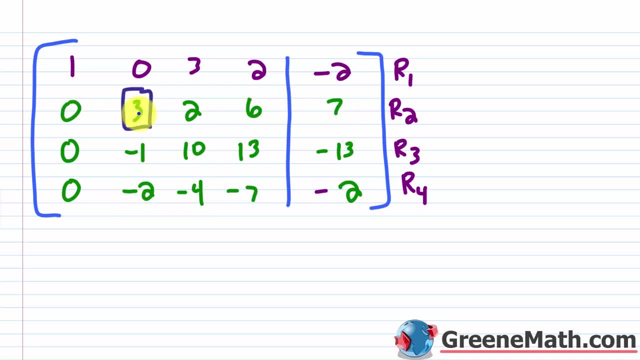 below, okay, so the easiest way to get a one in this position is to do this right. so I'm going to get here. I can multiply any row by a non-zero real number, so I'm just going to multiply this whole row, row two, by the reciprocal of three, because three times a third would give me one, okay, so 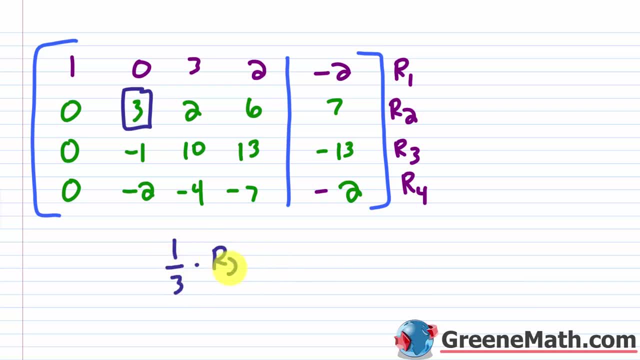 I'm going to multiply one third times row two. that's what I'm going to replace row two with. so this would be one, this would be two thirds, this would be six thirds, which is two, and this would be seven thirds. okay, so that's pretty quick, and now I want to get a zero here and I want to. 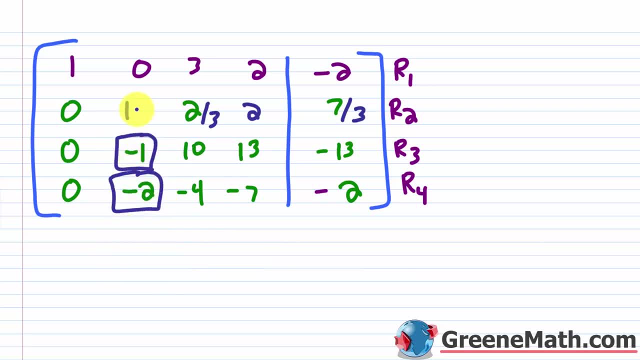 get a zero here. so I know the additive inverse of negative one is one. so again, I could multiply one times row two and add that to row three. that's what I could replace row three with if I want this to be a zero. and again, if I'm multiplying by one, it's just itself. so you can just erase that. 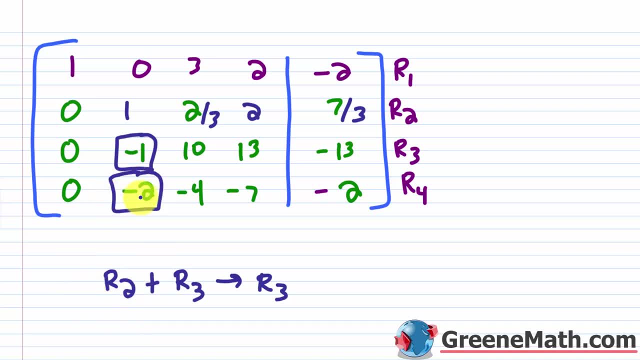 then for this one, the additive inverse of negative two is two. so I want to multiply two times row two and then add that to row 4. that's going to give me my new row 4, okay, so for this guy right here, I'm just going to add: 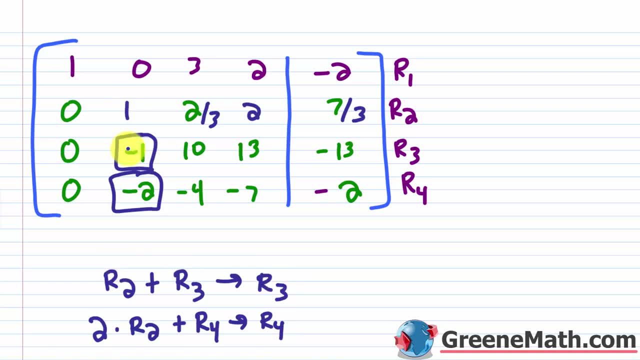 row 2 and row 3 and that's going to replace row 3. so 1 plus negative 1 is 0. then you would have 2 thirds plus 10. well, I know I could write this as over. I could multiply this by 3 over 3, so this: 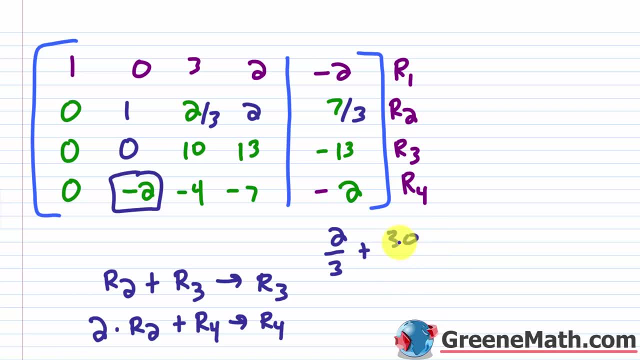 would be 30 thirds, and 30 plus 2 is 32. so this would be 32 thirds. so this would be 32 thirds. then I'd have 2 plus 13, which is 15, and then, lastly, I would have 7 thirds plus negative 13. 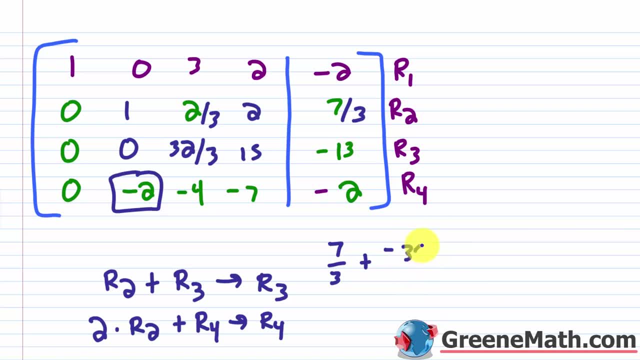 multiply this by 3 over 3. you would get 39 there over 3. so negative 39 thirds. so negative 39 plus 7 would be negative 32. so this would be negative 32 thirds. okay, so let's erase this and this. this one's done. so now let me work on this row. here again, I want that to be a 0, so I'm going. 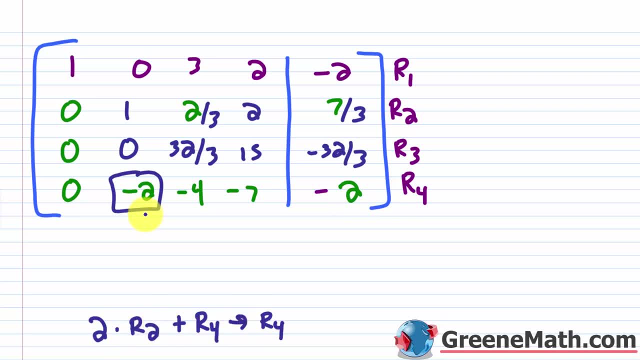 to multiply 2 times row 2, add the result to row 4. that's what I'm going to replace row 4 with. so we know this is going to be a 0, 2 thirds times 2 is 4 thirds then, plus negative 4. 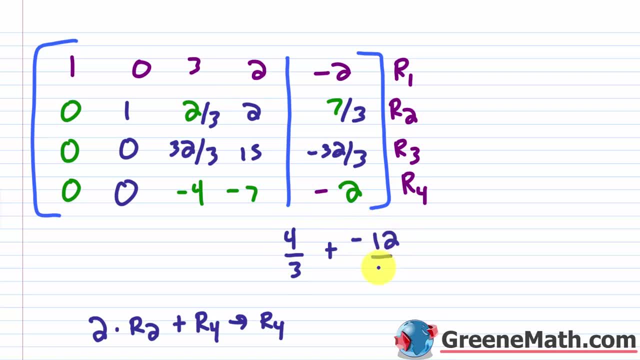 multiply this by 3 over 3. you get negative 12 thirds- 4 plus negative 12 thirds. 12 is negative 8. so this is going to be negative 8 thirds. okay, then the next one is going to be 2 times 2, which is 4. 4 plus negative 7 is negative 3. 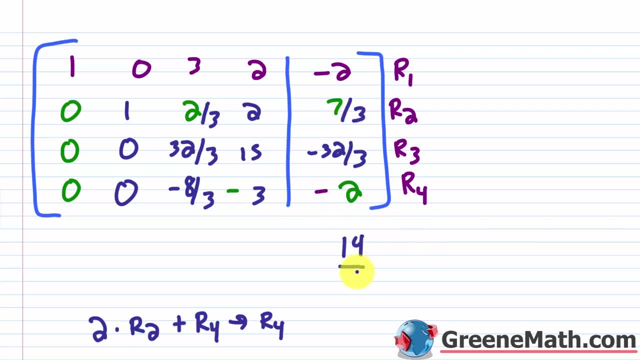 then the last one's, 2 times 7 thirds, which is 14 thirds. then plus negative 2, which I'll write as negative, 6 over 3. so 14 minus 6 is going to be 8. so this would be 8 thirds. so I'll put this as: 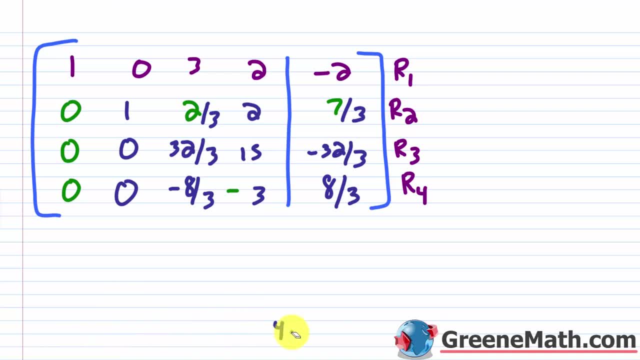 8 thirds. okay, so let me erase this. so far, so good. so now I want to get started. okay, these two columns to the left are done. I want this to be a 1, so you already know the deal. I'm going to multiply row 3 by 3 over 32, and this gets easier as we move on, because I don't. 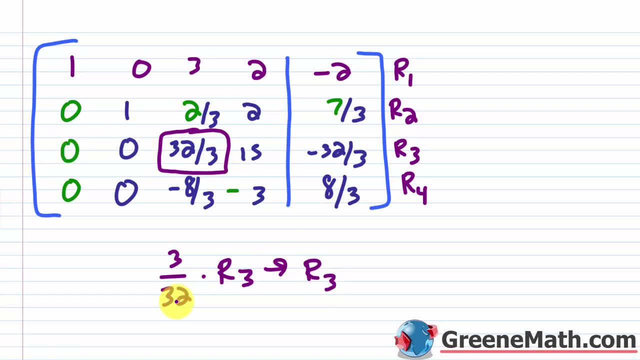 have to worry about this stuff over here. this is 0 and this is 0, so multiplying that by the reciprocal doesn't do anything right. it's still 0. this is going to be 1. we already know that. so really, the only calculation I have to do is 15 times 3 over 32, which is going to be 45 over 32. 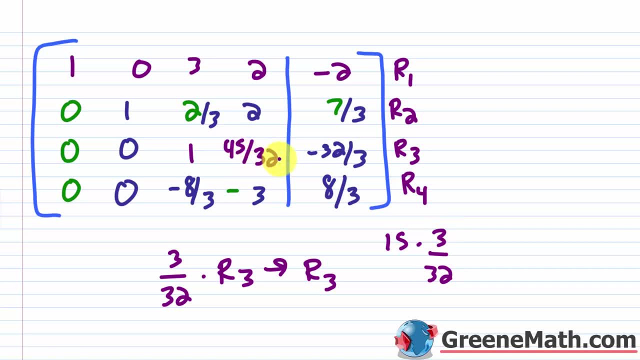 and then you would have your negative 32 over 3 times 3 over 32. this cancels, and this cancels. you get negative 1. so this is negative 1 here. okay, so let's erase this. okay, so let's think about getting a 0 here, here and here. okay, so three different things we want to do again in each. 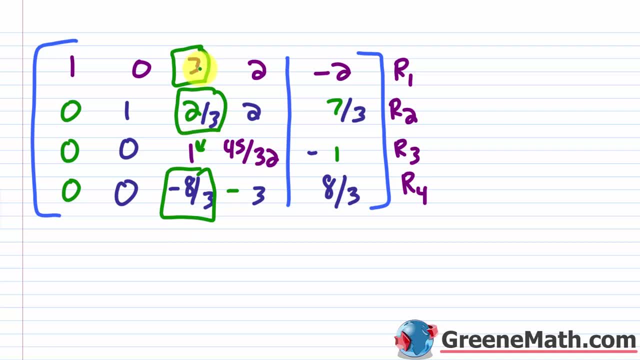 case, because I've got a 1 there. think about what the additive inverse is of what you're trying to make into a 0, and then you're going to have a negative 1 here and then you're going to have a negative 2. so you're going to multiply that by that row with the 1 in it and then add that to. 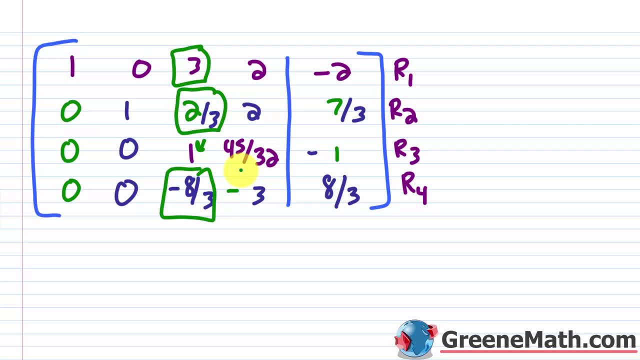 the current row, that you're trying to make that into a 0. I know I said a lot there, but basically, if you think about this for row 1, I'm trying to make this 3 into a 0, so I'm going to multiply row. 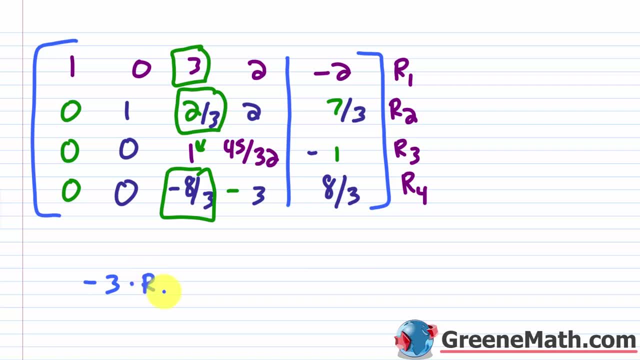 3 by negative 3, the additive inverse of that. add the result to row 1. okay, so that's going to take care of that. that's what I'm going to replace row 1 with same concept as we move on. so for row 2. 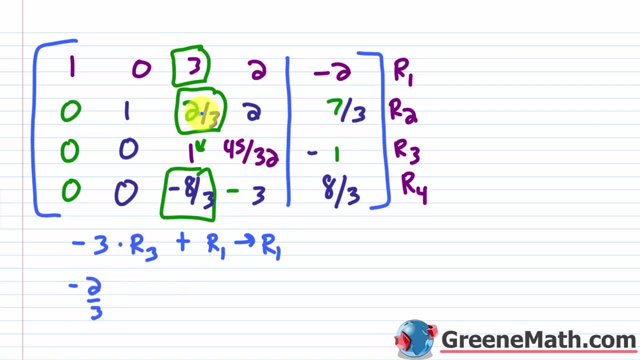 I'm going to multiply negative two-thirds, which is the additive inverse of two-thirds times row 3. okay, that 1 in row 3 plus row 2, that's what I'm going to replace row 2 with. and then, lastly, for row 4, I'm going to take positive eight-thirds. 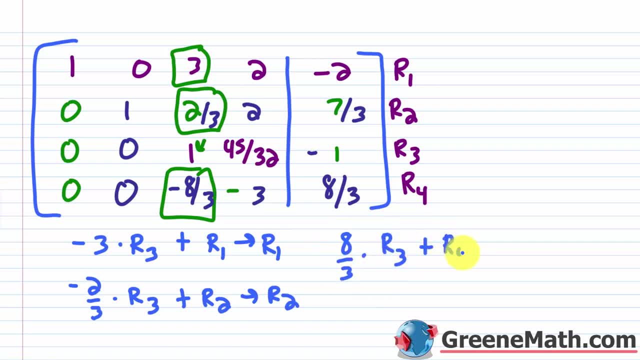 multiply it by row 3. add the result to row 4. that's what I'm going to replace row 4 with, all right, so let's do these one at a time. so let's start with this kind of row 1 here. so I want. 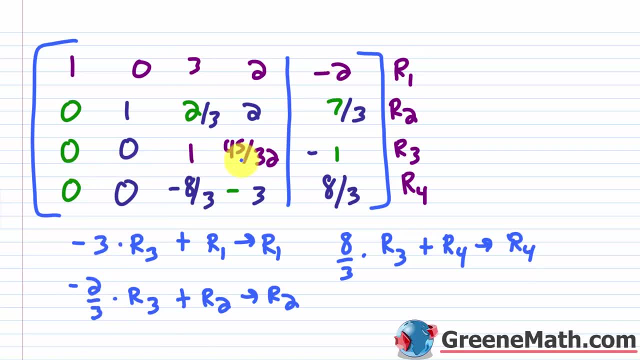 negative 3 times this row 3. okay, I'm going to add the result to row 3 and then I'm going to add the result to row 1 now, because these two guys here are zeros. I don't need to worry about it. zero times. 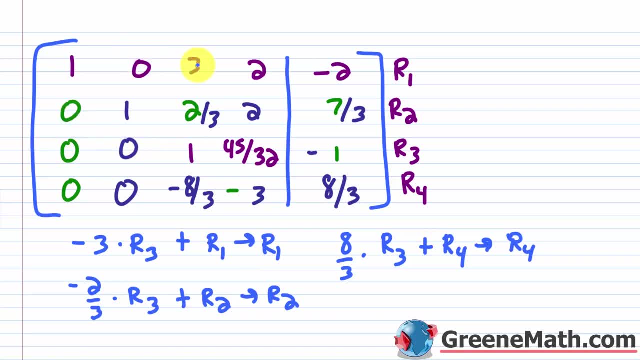 anything is zero. adding zero to something doesn't change it. I know this would be zero, I don't even need to worry about that. I just have to do the calculation for these two. so I would start here with this kind of 45 over 32 and I would multiply it by this negative 3, okay, by this negative 3, and. 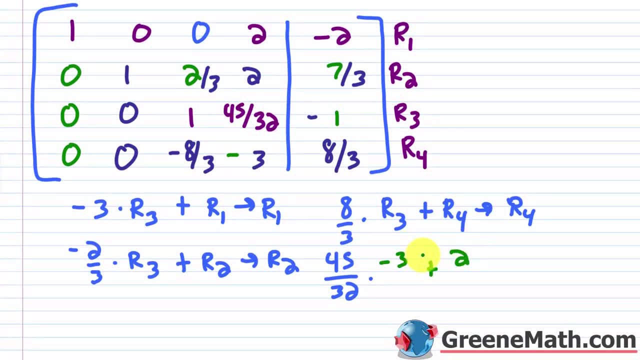 I would add to this this value of 2.. okay, so that's one of them that I have to do. then the other one times negative 3, and then I'm going to add to that negative 2, so let's kind of slide down here. 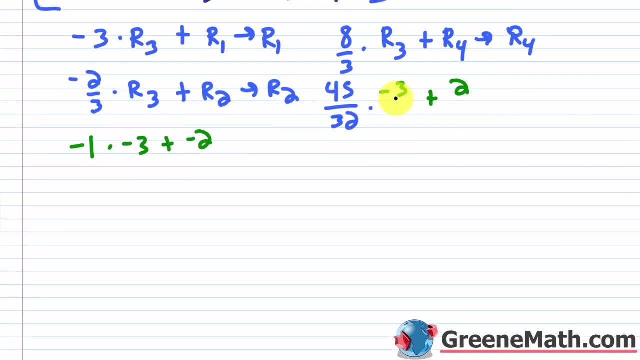 and do this and we'll come back up. so 45 times negative 3 is negative 135 and this will be over 32. then plus for 2, to get a common denominator, I would write it as 64 over 32. so if I sum these: 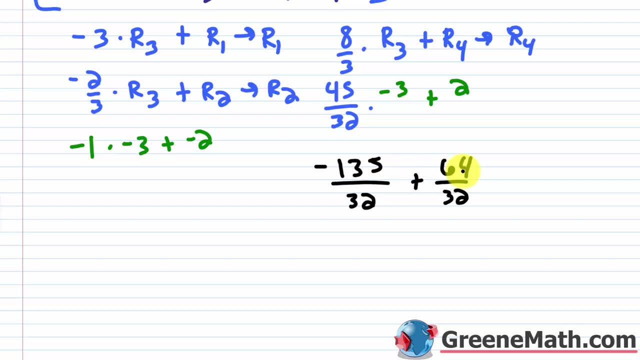 negative 135 plus 64 is going to be negative 71, so this would be negative 71 over 32. okay, so for negative 1 times negative, 3 is 3, right positive 3 and positive 3 plus negative 2 is positive 1. 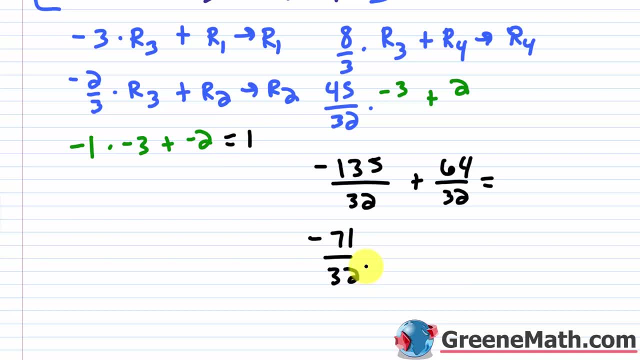 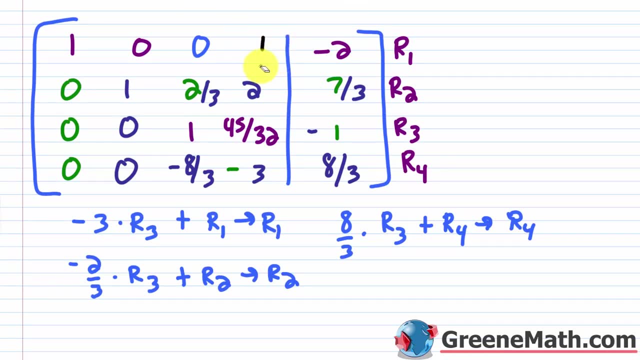 so I'm going to have negative 71 over 32 and I'm going to have positive 1, so let's erase this. so we'll put this as negative 71 over 32. let me make that better. so negative 71 over 32 and then. 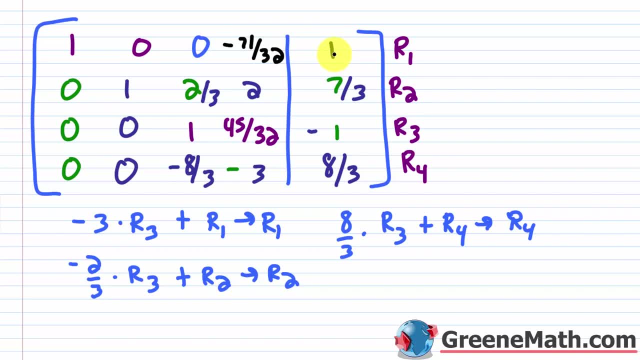 again. this was positive 1. okay, so now I can erase this. this part's done. let me kind of slide this up, so now let's work on this one. so I know that this, right here again, I'm multiplying negative two-thirds times row 3. so this and this are not affected. this is going to be a 0. this, right here, I would have negative. 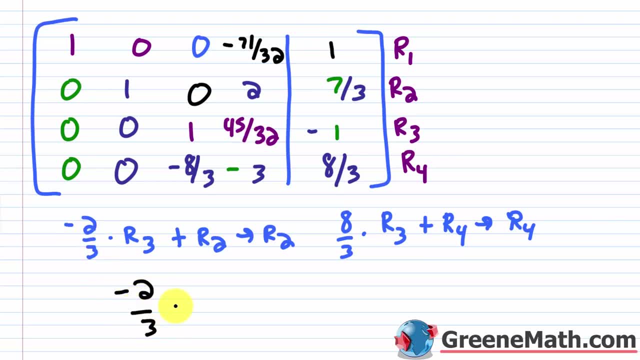 two-thirds times. so negative. two-thirds times 45 over 32, and then the result of that would be added to 2. so let's figure out what this is. so this cancels with this and gives me a 16 down here. this cancels with this and gives me a 15 here. so this is negative 15 over. 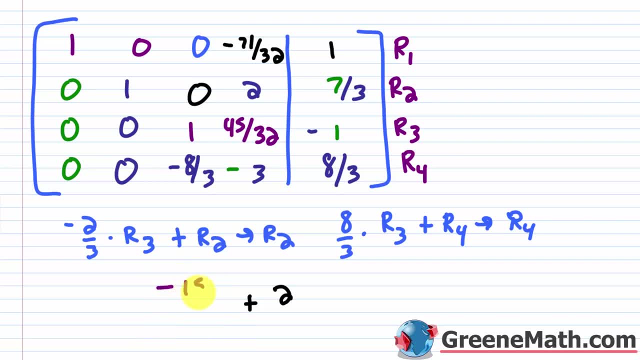 16. so negative 15 over 16. to get a common denominator going, I'm going to say: this is 32 over 16 and then 32 minus 15 is 17. so this would be 17 over 16. so that's what I'm going to put. 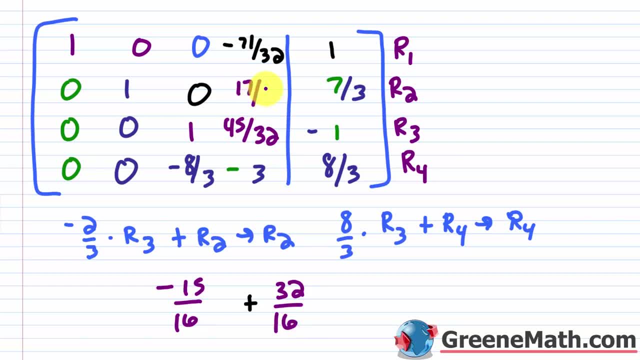 right. here it's going to be again 17 over 16. all right, and then one more. to do so, I'm going to multiply negative two-thirds times negative 1, so negative two-thirds times negative 1, which would just be two-thirds. then I'm going to add the results to this seven-thirds here. okay, so two plus seven is nine. 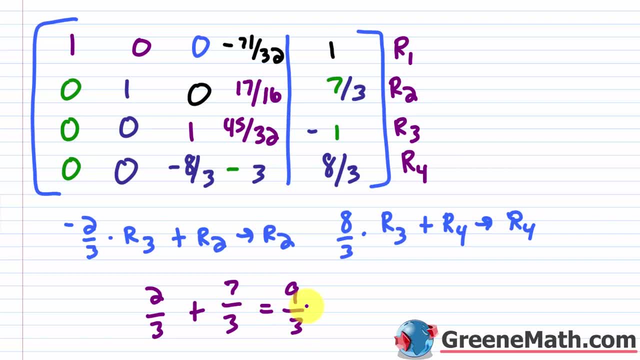 so this would be nine over three, which is three, so I'm going to replace this with a three. okay, so let's erase this one, and now we're just going to work on this one. so I've got eight-thirds times row three plus row four. so if I go through again this one and this one, it's not going to change. 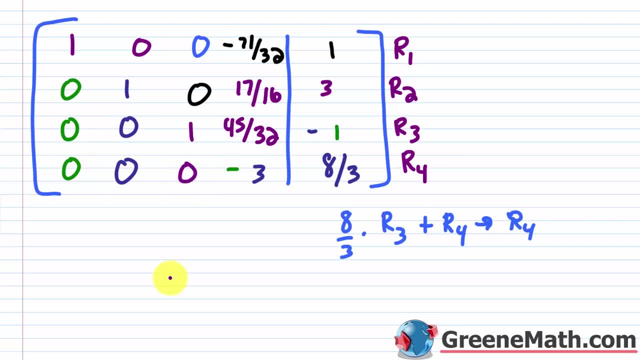 these. this guy's going to turn into a zero. so what I want to do is: eight-thirds times 45 over two. so this cancels with this and gives me a four. this cancels with this and gives me a 15. so you have 15 fourths plus negative three. so 15 fourths. you can go ahead and just say minus three. 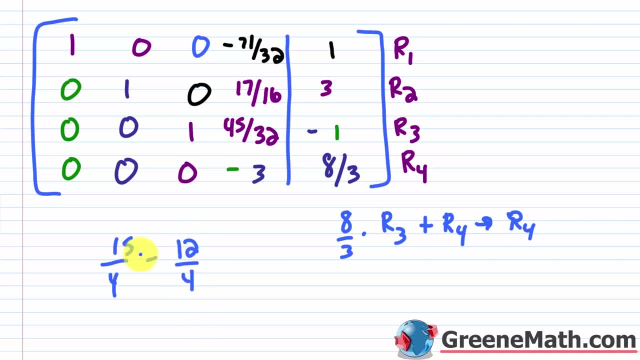 three is 12 over four. 15 minus 12 is three, so this is just three-fourths, three-fourths, all right. then we want to do eight-thirds times negative one, which is just negative eight-thirds, and then we want to go plus eight-thirds, which is obviously going to give us zero. so this will be zero here. all right, so not. 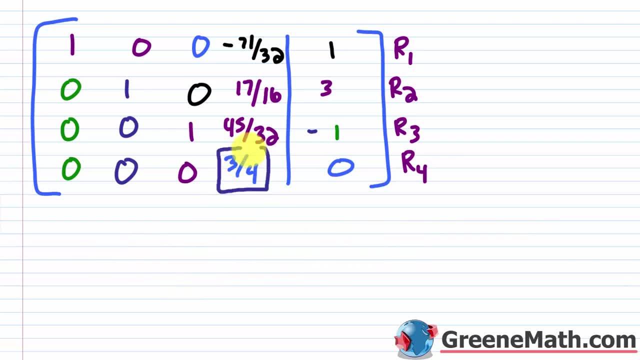 much left, so we want to get a one here now, and to do that I can just multiply row four by four-thirds. obviously you can see that x sub four is going to be zero, right, because when I multiply this by four-thirds, this by four-thirds, this by four-thirds and this by four-thirds, it's all going to stay. 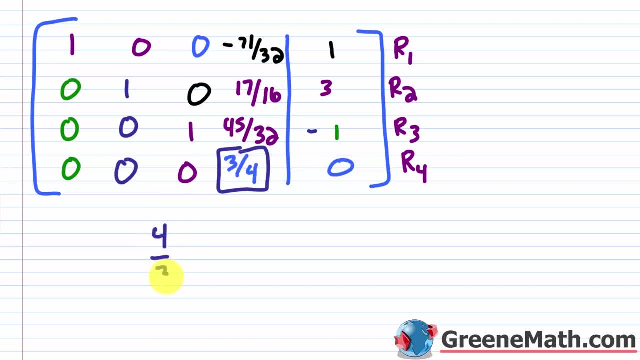 zero. this is going to change into a one, right? so four-thirds times. row four is what I'm going to replace row four with, so this will just be one. okay, all right, now I'll want to zero here, here and here. so to get the zero here, I'm going to multiply row four by negative 45 over 32. add the result to 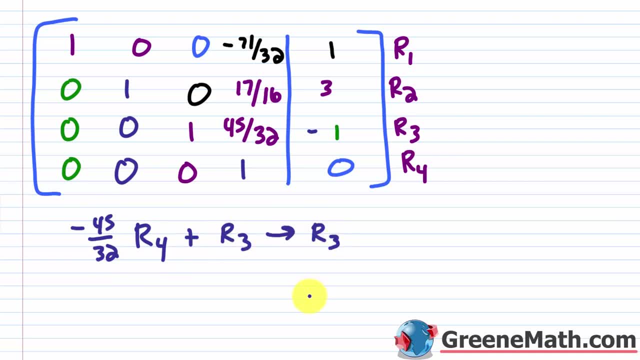 row three. again, that's what I'm going to replace row three with. and then I'm going to multiply negative 17 over 16 times row four. add the result to row two. that's what I'm going to replace row two. and then, lastly, I'm going to multiply 71 over 32 times row four. add the result to row one. that's. 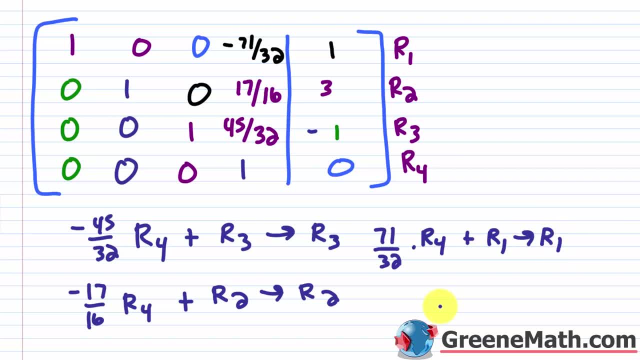 what I'm going to replace row one with now. before I do anything, you might want to notice that this is a zero, this is a zero, this is a zero and this is a zero. so, in every case, whatever this number is, it doesn't matter when it multiplies these guys by zero and I add it to whatever row. 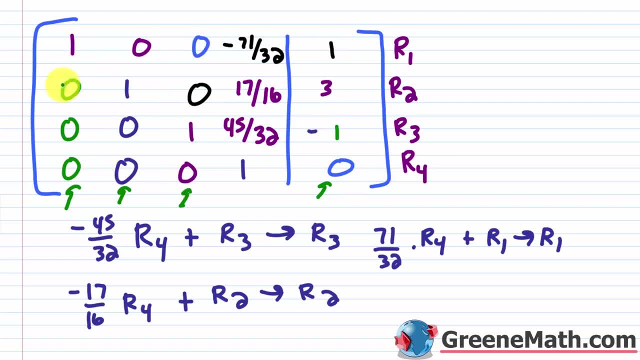 it is, it doesn't change. so none of these entries are going to change anywhere, except for here, here and here, and in every case I'm adding exactly what I need to make them into a zero. so I can just go ahead and put zero, zero, zero and say: 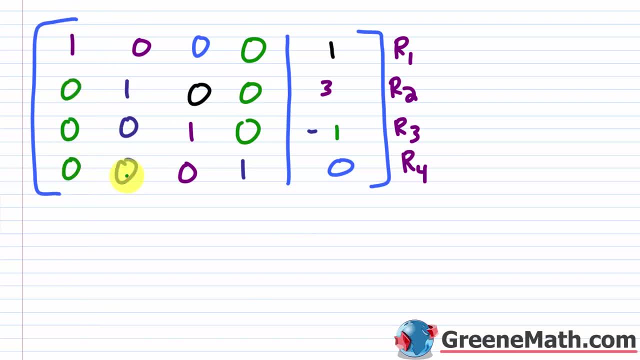 we have our solution. so remember it's the coefficients for x sub one, then x sub two, then x sub three, then x sub four. so for x sub one it's going to be one, for x sub two it's going to be three. for x sub three it's going to be negative one. 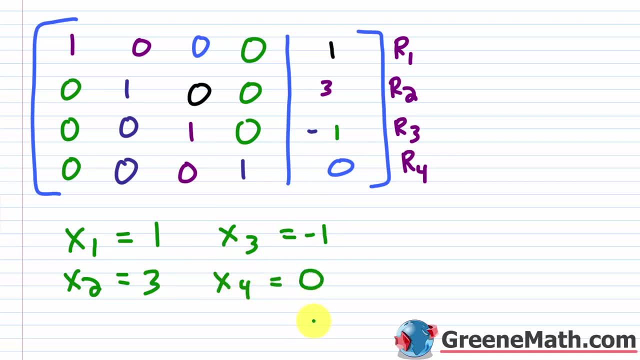 and for x sub four it's going to be zero. so again, in this particular case, we just so happen to get x sub one through x sub four. but if you add w, x, y and z, remember the leftmost column will be w, then x, then y, then z. it goes in alphabetical order with subscripts: you go one, two, three and four. you go in. numerical order.